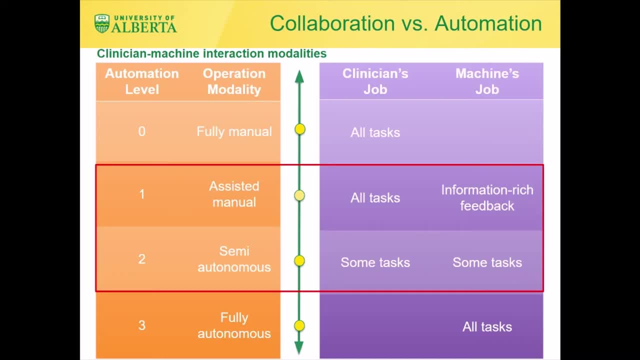 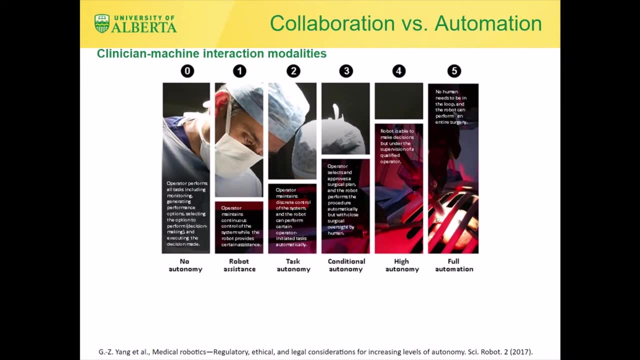 and enables the clinician to focus on the more critical tasks In terms of the staircase of increasing autonomy shown in the paper at the bottom of this page. I'm going to focus on the mid-levels of robot autonomy, where there is some type of shared control between the clinician and the robot. 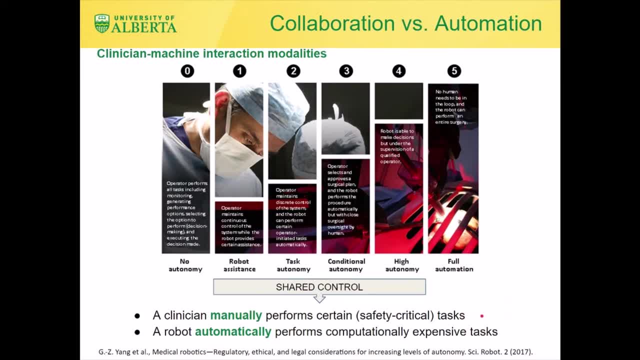 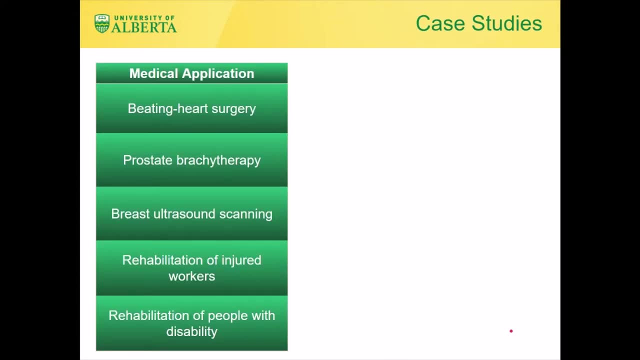 The clinician manually performs the tasks, performs certain tasks that are safety-critical, while the robot automatically performs tasks that are computationally expensive in a way that extends the abilities of the clinician and improves the outcomes for the patient, As shown on the left side. I will present several case studies of shared control between a clinician and a robot. 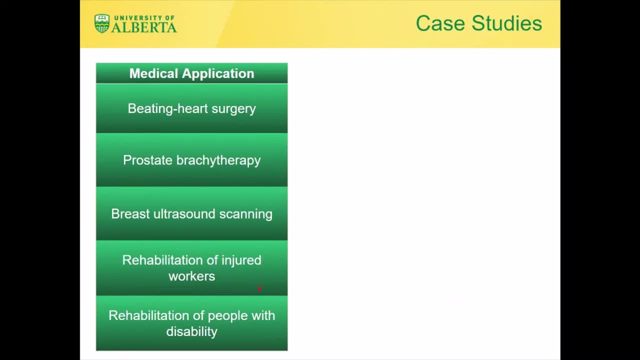 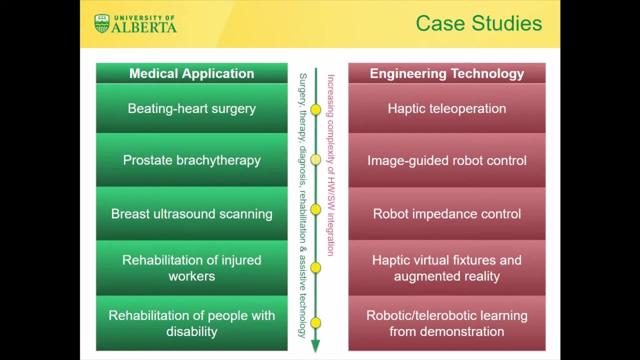 spanning surgery, therapy, diagnosis, rehabilitation and assistive technology. I will also talk about the engineering technology shown on the right side that were used to address these clinical challenges. Let me start with the system-controlled challenges associated with beating heart surgery. 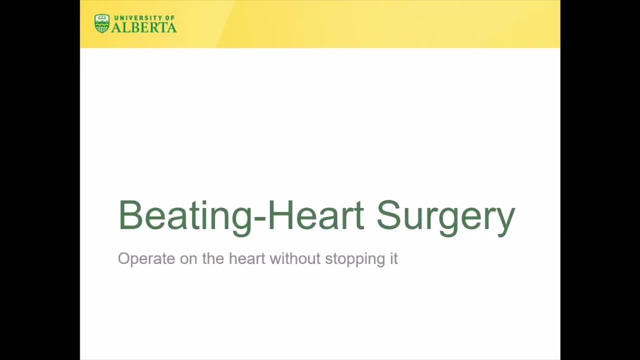 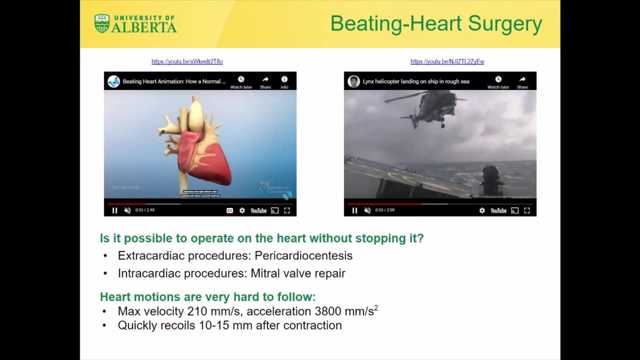 In beating heart surgery, the goal is to operate on the heart without stopping it. The heart has fast motions that are very hard for the human hand to follow. Is it possible to operate on the heart without stopping it as far as an extracardiac procedure such as pericardial synthesis? 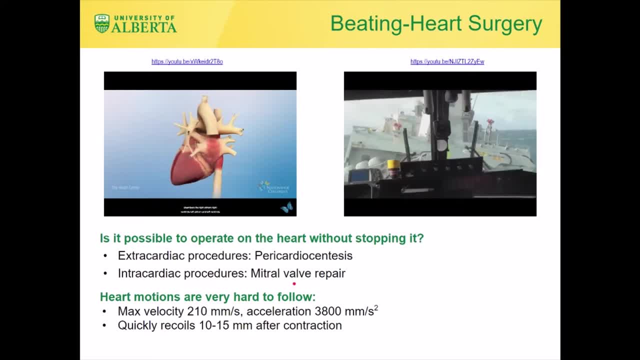 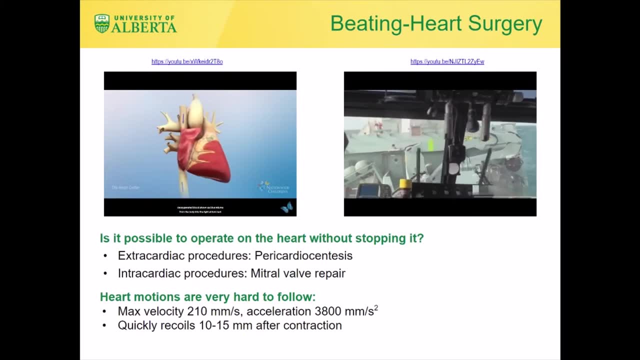 or an intracardiac procedure such as mitral valve repairs is concerned. Operating on the heart as it beats is similar to landing a helicopter on the deck of a ship in choppy waters. To avoid collision with the ship, the pilot should control the distance between the helicopter and the ship. 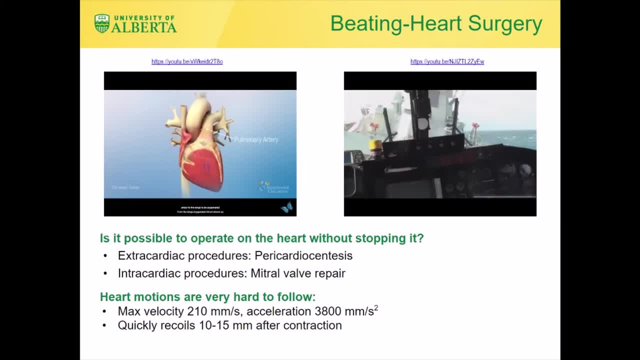 using position commands read from a joystick. In a similar way, the surgeon needs to be able to control the distance between the tip of the surgical instrument and the heart tissue using position commands read from the surgeon's console, Doing such motion compensation in an unassisted and manual way. 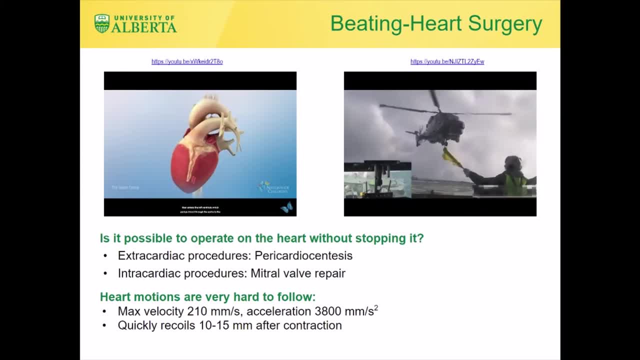 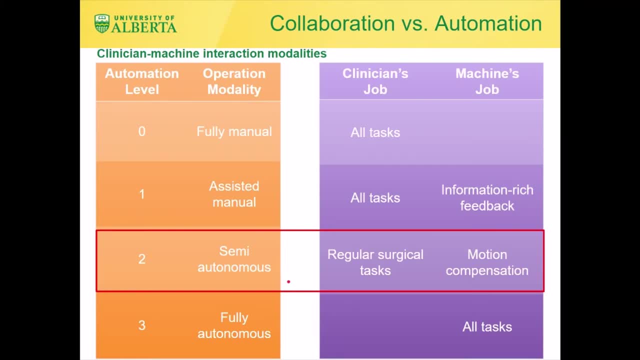 requires very high level of mental focus and motor skills and is next to impossible to do for a human. However, this is where robot semi-autonomy and human-robot collaboration can come to the rescue. A shared control scheme can facilitate beating heart surgery if it delegates the task of motion compensation to the robot. 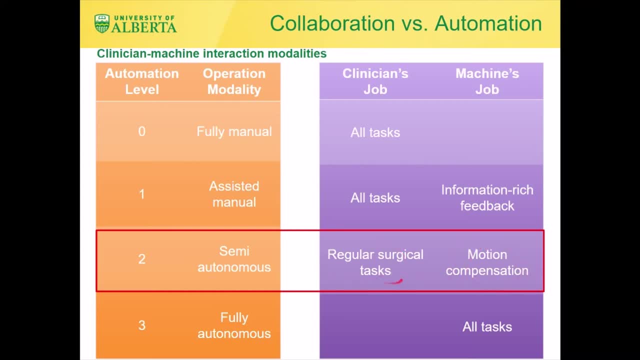 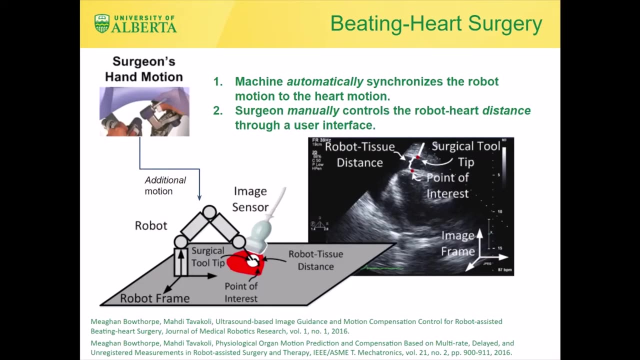 so that the surgeon can focus on performing regular surgical tasks, as if the heart has been arrested and doesn't move. This is how we envisioned the shared robot control system to work. Ultrasound images are used to collect the position of the heart tissue, the position of the tool and therefore, the distance between the two. 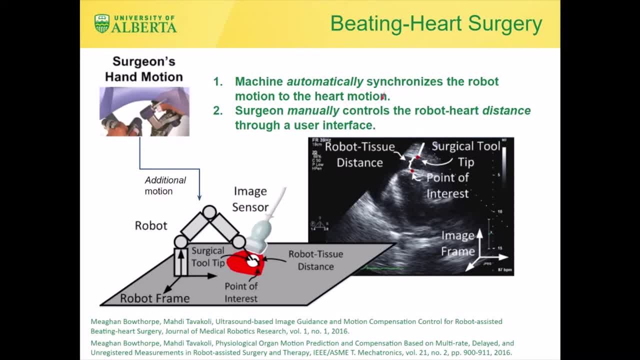 The machine automatically synchronizes the robot motion to the heart motion by making the distance between them follow the surgeon's hand motions. In this way, even when the surgeon's hand does not move, the surgical tool is moved by the robot in a dance with the heart tissue. 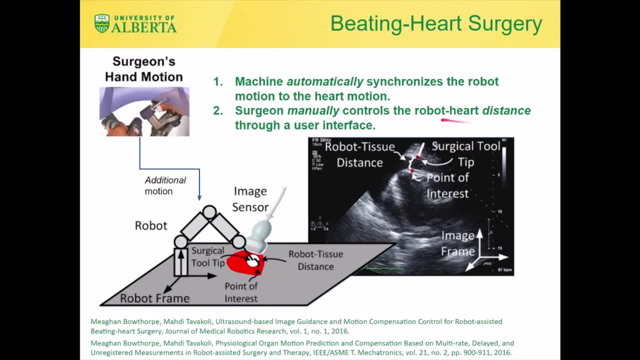 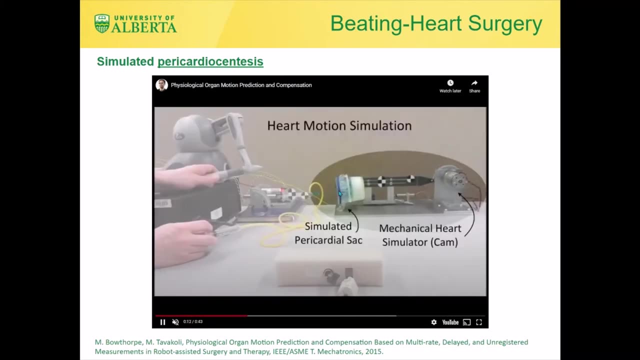 The surgeon then manually controls this robot heart distance through the user interface so that the surgical task can be performed as if the heart does not beat, Skipping the details of feedback control. this is how the system works. We have a mechanical heart simulator with a sac of fluid around the simulated heart. 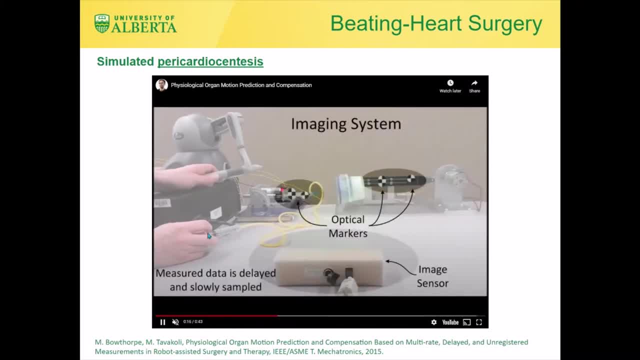 to be drained, similar to what happens in pericardial synthesis In the uncompensated or unassisted mode. the user has to control the user interface such that the tip of the syringe moves in synchrony with the heart and at the same time properly penetrates the fluid sac to be able to withdraw the fluid. 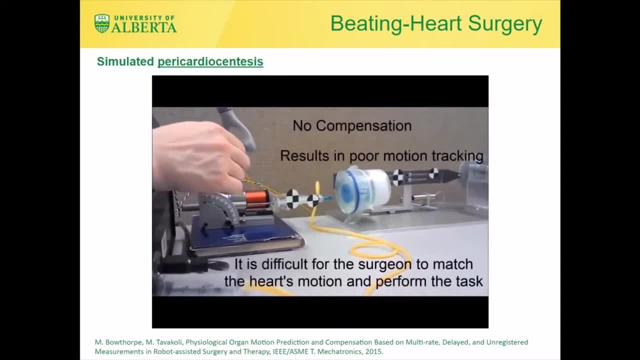 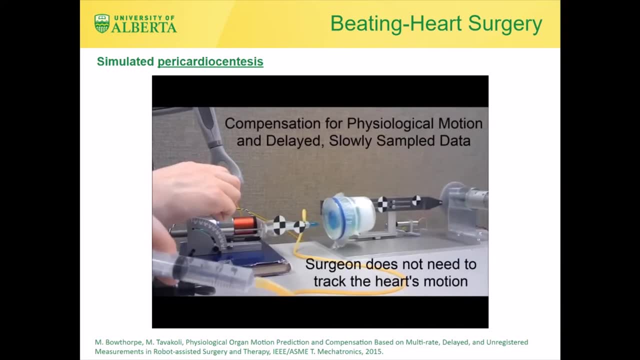 This job is next impossible for the user In the compensated or assisted mode. the user's hand is relatively steady, as it only provides the reference value for the syringe to heart distance and the robot automatically takes care of the position. control of the syringe. 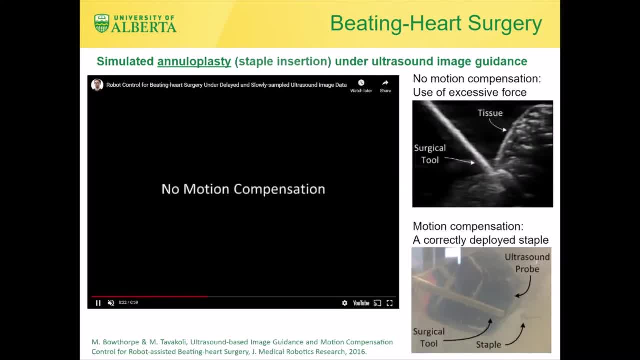 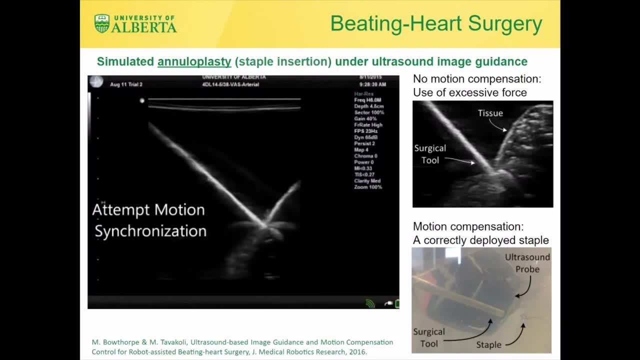 for good motion, compensation For the case of annual opacity for mitral valve repair. we focus on the stapling task using the same mechanical heart simulator, but under live ultrasound imaging. Again, without robotic assistance, it is almost impossible for the user to move the tool in a dance with the heart tissue. 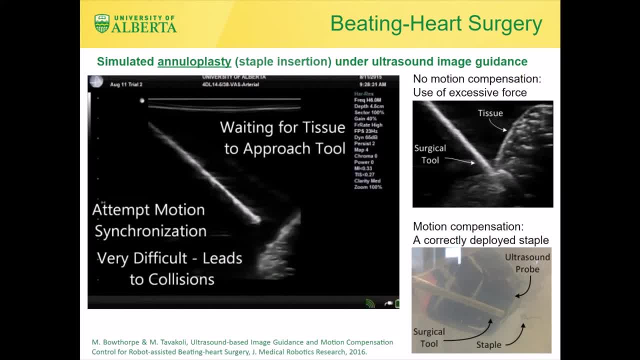 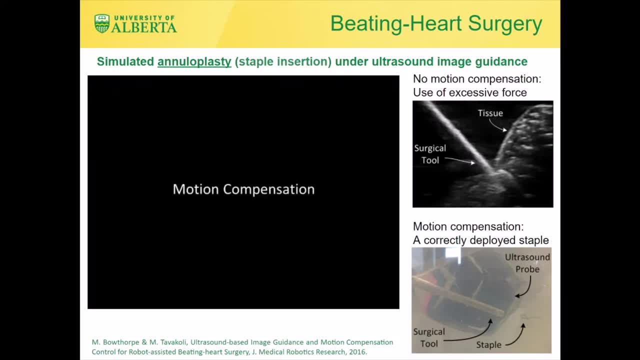 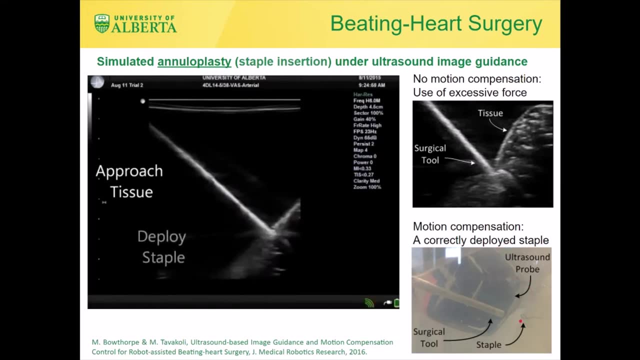 and, at the same time, deploy the staple at the correct distance and time. With robotic motion compensation, however, the user simply focuses on controlling the distance between the tool tip and the heart tissue through joystick position commands and is able to deploy the staple successfully in 100% of times. 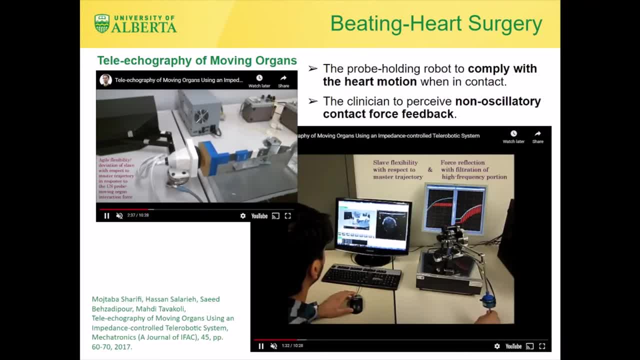 A related application is tele-echocardiography, when the organ to be imaged has semi-periodic movements due to respiration or heartbeat. With robotic motion compensation, the sonographer will be able to focus on lateral motions of the probe that are tangent to the tissue surface. 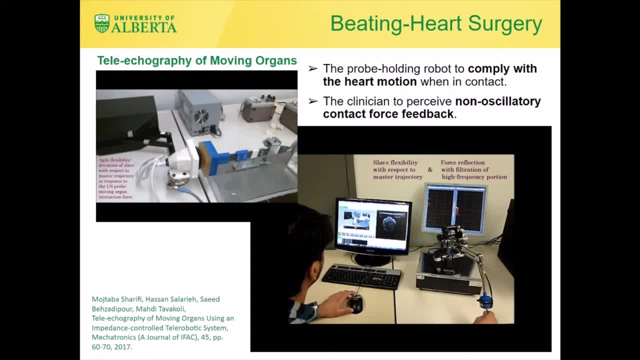 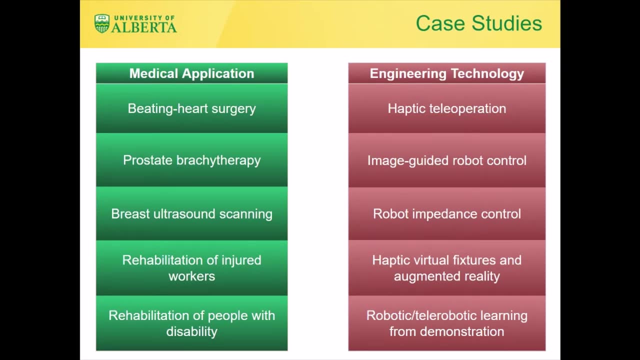 because the robot control system takes care of appropriately moving the probe in the direction normal to tissue, such that the probe tissue contact force is held steady for good and consistent image quality. The next case study where some sort of shared control between the clinician and the machine can result in better outcomes. 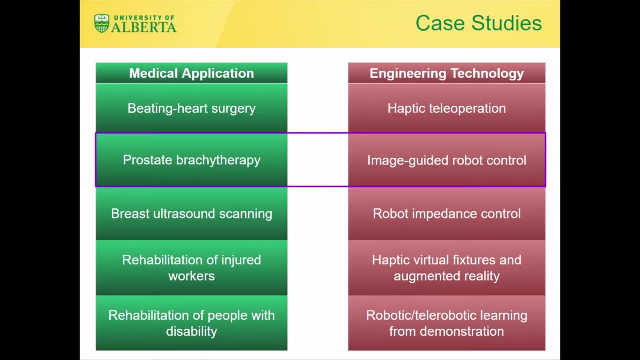 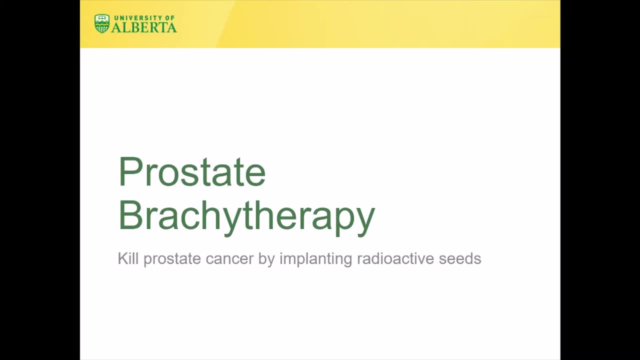 is prostate brachytherapy under ultrasound image guidance. In prostate brachytherapy the goal is to kill the prostate cancer by implanting radioactive seeds in or around the tumor. In prostate brachytherapy, long and hollow needles carrying radioactive seeds. 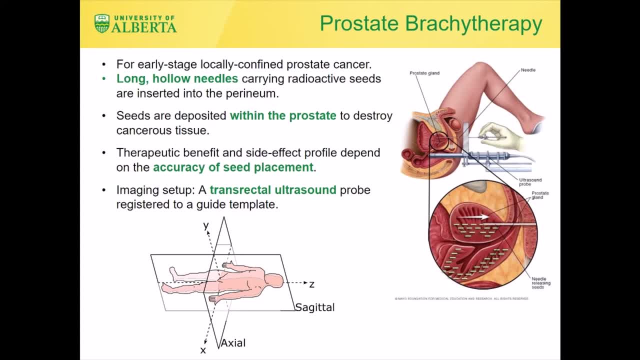 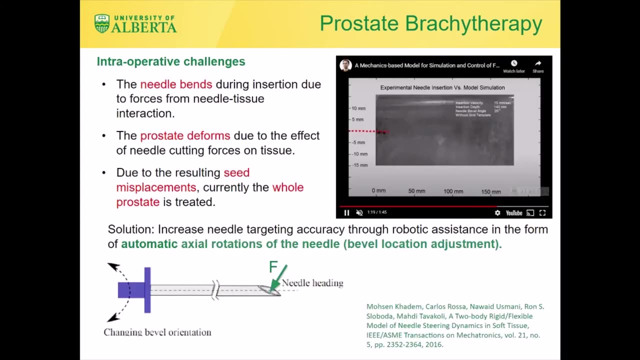 are inserted into the prostate under transrectal ultrasound imaging. Once needles reach target locations, these seeds are deposited within the prostate to destroy the cancer's tissue over time, Intraoperatively. the issue is that the needles bend during insertion due to forces from needle-tissue interaction. 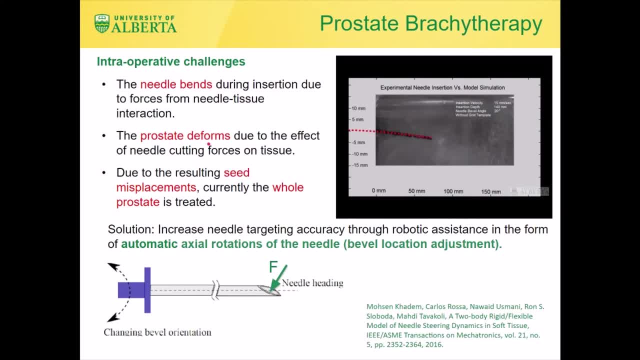 and also the prostate deforms due to the effect of needle-cutting forces. This results in seed misplacement, which undermines the effectiveness of the procedure. Fortunately, by axially rotating the needle, it is possible to control the needle path. However, needles have poor visibility in ultrasound images. 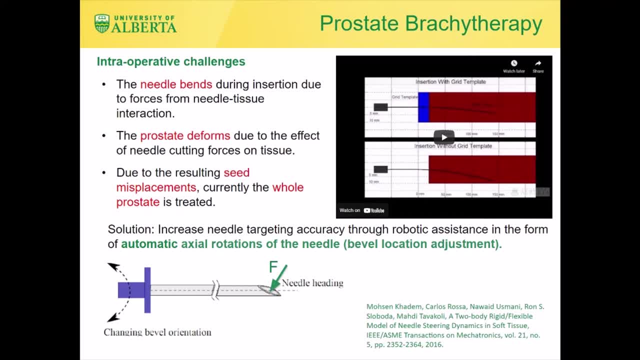 and the needle is a continuum robot with non-holonomic constraints, making it difficult for the surgeon to know at what depth of needle insertion the needle should be rotated and by how much. This is where we can resort to intelligent shared control of needles. 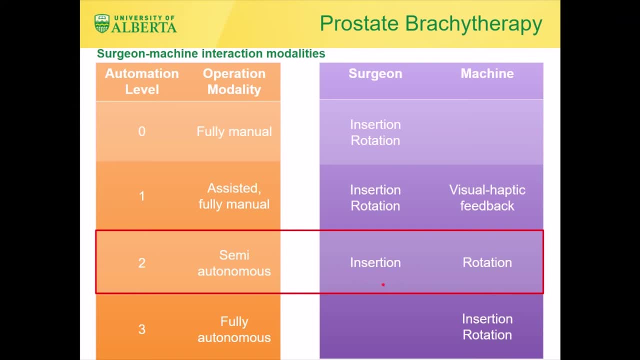 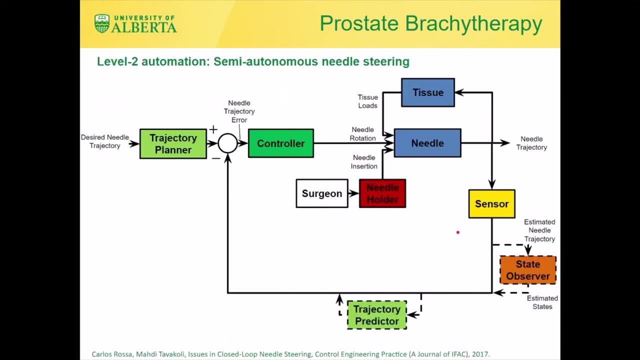 Needle insertion, which is a safety-critical task, can be left in the hand of the surgeon, while needle rotation can get delegated to the machine. This is because needle rotation is best done using sensors that estimate the needle tip position. state observers that estimate the needle tip orientation. 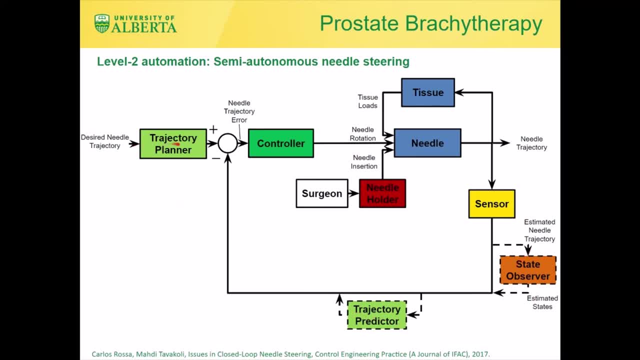 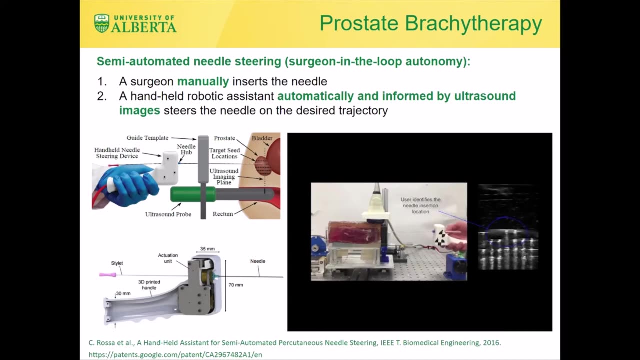 trajectory predictors and trajectory planners that take into account the non-holonomic constraints of the needle motion, and a controller that is informed by the coupled needle-tissue dynamical model. This is how the semi-automated needle-steering system works. A surgeon manually inserts the needle using a handheld robotic assistant. 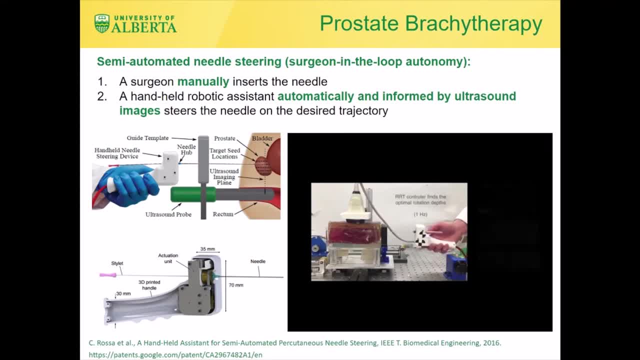 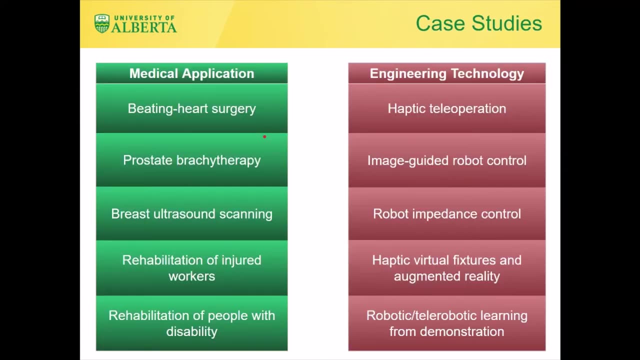 that holds the needle, while the computer-controlled assistant automatically, and informed by ultrasound images and control and path planning algorithms, rotates the needle appropriately to steer it on the desired trajectory. Another case study for sharing the medical robot control between a computer and a clinician involves breast ultrasound scanning. 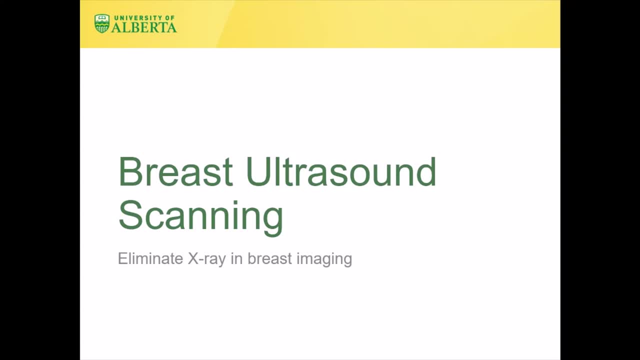 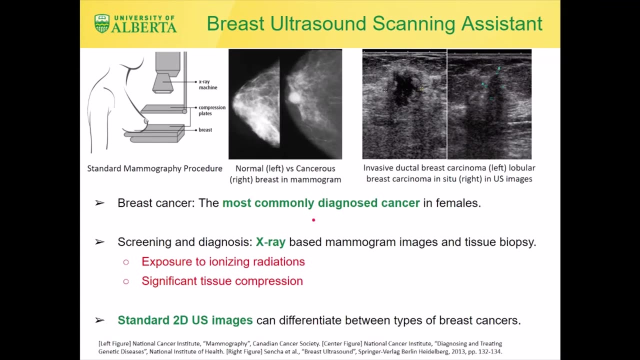 With breast ultrasound scanning. the goal is to eliminate X-ray in breast imaging. Using X-ray-based mammogram images for breast cancer screening and diagnosis poses two challenges: exposure to ionizing radiations and significant tissue compression. With ultrasound imaging, we are able to avoid both problems. 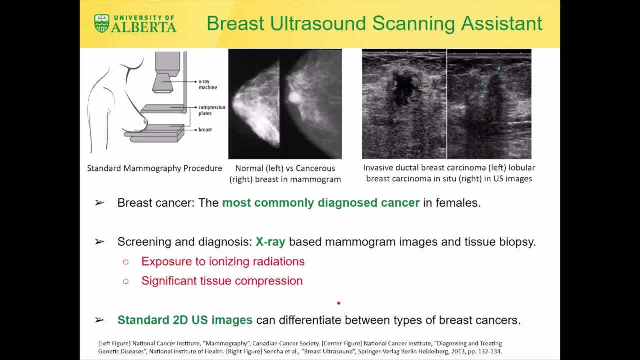 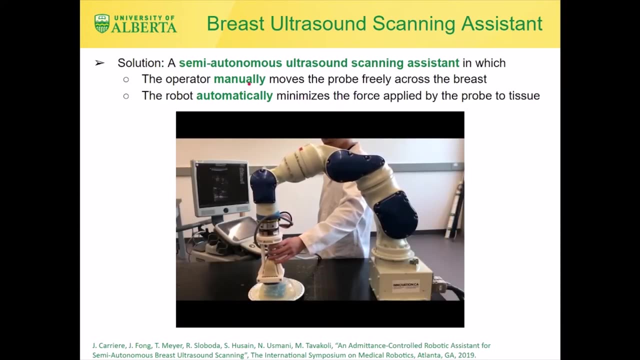 while visualizing breast cancers. Minimally deforming the breast during imaging makes it easier to do the image-guided surgical planning for tumor removal. later We've developed a semi-autonomous ultrasound scanning assistant in which the operator manually moves the probe freely across the breast. 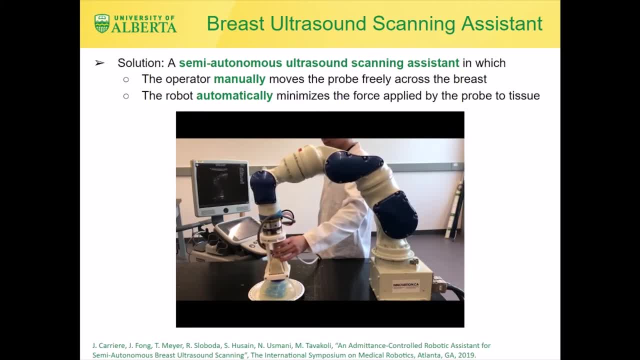 while the robot automatically controls the force applied by the probe to tissue. Informed by real-time feedback of ultrasound image quality, the robotic system can minimize the forces applied to the breast for causing minimum tissue deformation, while ensuring consistent image quality. This is yet another way to leverage intelligent semi-autonomous robot control. 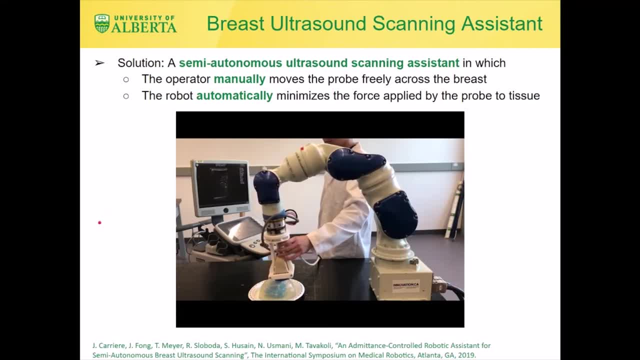 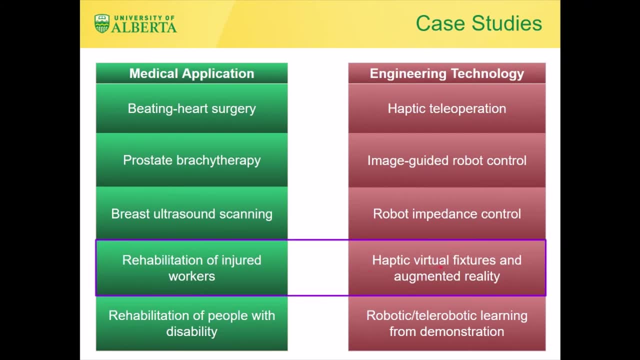 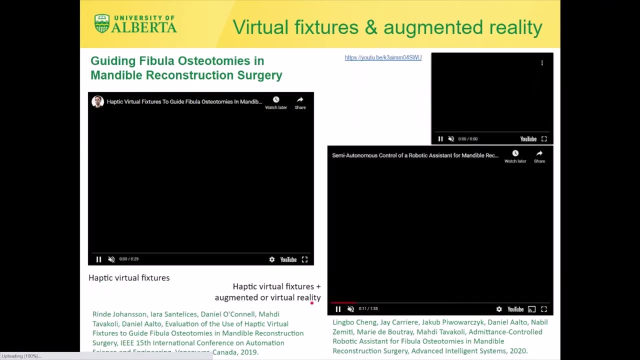 to make the clinician's task simpler while improving the procedure outcomes. One other way to incorporate intelligence into medical robotic systems is through haptic virtual fixtures and augmented vision, such that information-rich feedback is provided to the user. We've developed a system that generates haptic virtual fixtures. 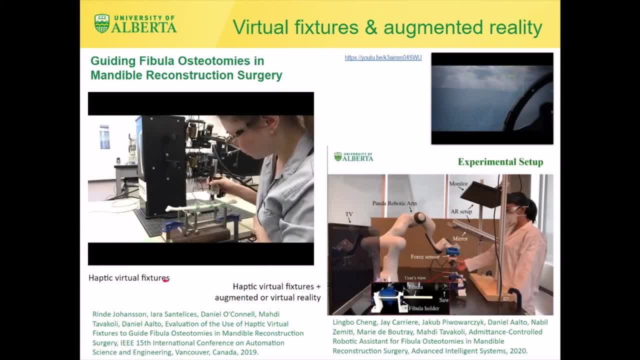 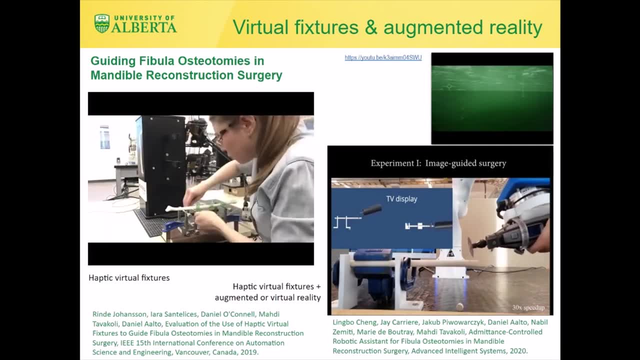 to guide the user's hand in CT-guided mandible reconstruction surgeries. The haptic virtual fixtures ensure that the bone is cut at the correct locations and correct angles. We've then added augmented reality so that not only the user's hand is guided toward the correct bone-cutting planes. 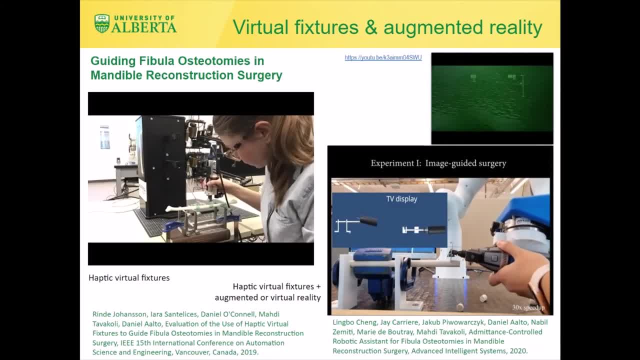 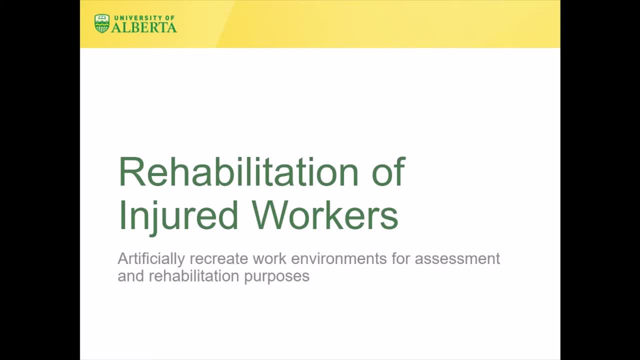 but also those planes are visually presented to the user as floating in 3D space. Haptic virtual fixtures and augmented reality can be used for rehabilitation of injured or disabled workers. in order to artificially recreate work environments for assessment and rehabilitation purposes, Typically, an injured worker goes through a functional capacity evaluation. 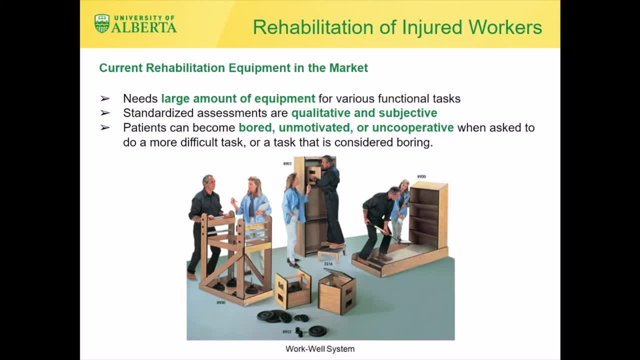 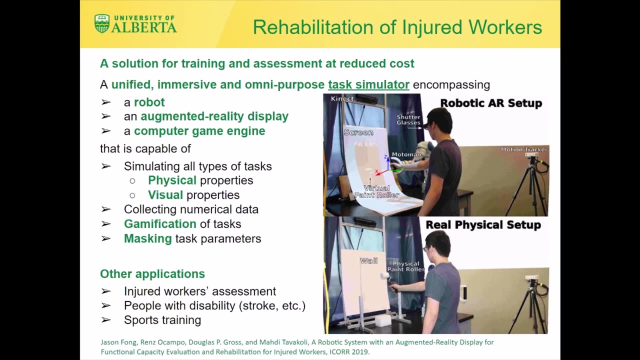 based on a standard set of workplace tasks that require large amounts of equipment and space to house them. In addition, the standardized assessments are qualitative and subjective, and patients can become bored or unmotivated in this process, Much like how a flight simulator recreates both the dynamics of flying an airplane. 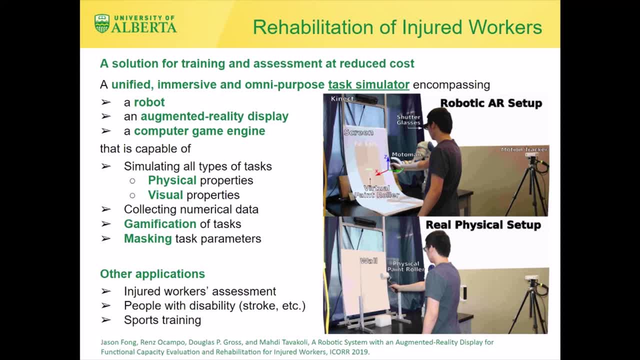 and the scenes viewed from the cockpit. we've developed a task simulator encompassing a robot, an augmented reality display and a computer game engine to create the haptic effects of performing a physical task In this way- both the physical and visual properties. 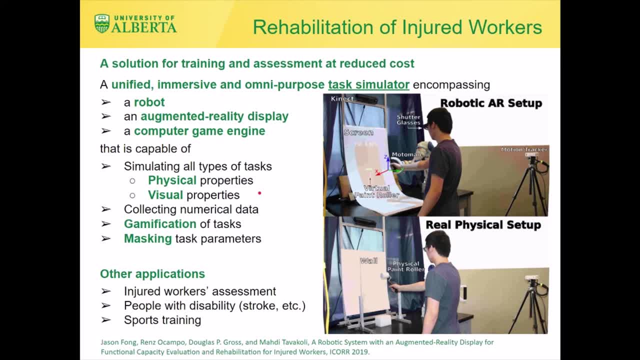 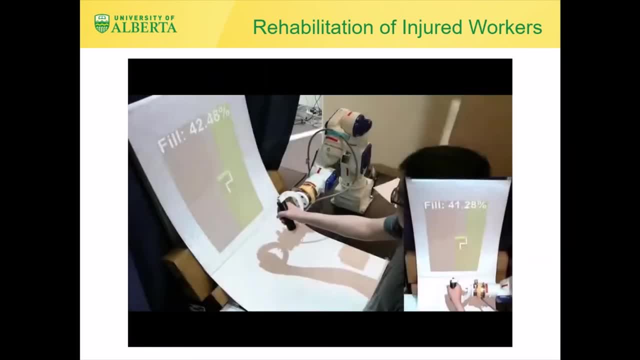 of a wide range of tasks can be simulated using the same system. When the 3D view is on, the user in this wall painting task will both see a wall in 3D using the projection mapping augmented reality system and feel it using the robotic manipulator. 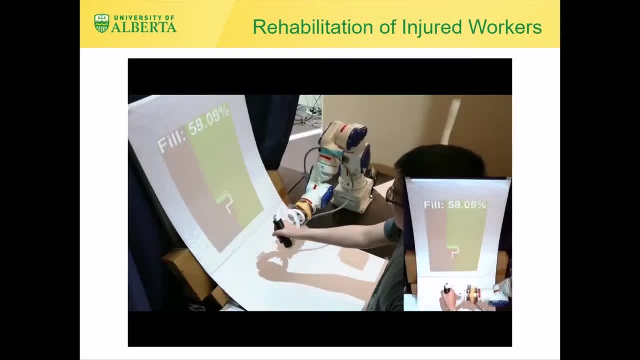 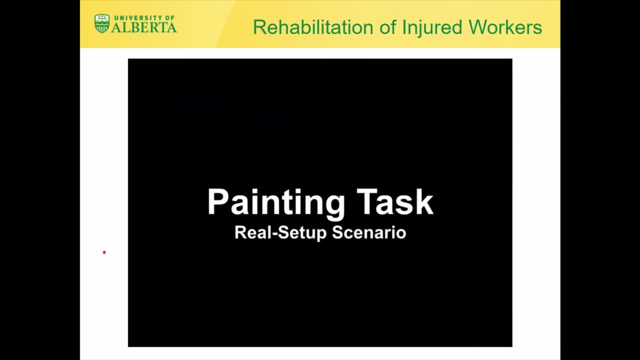 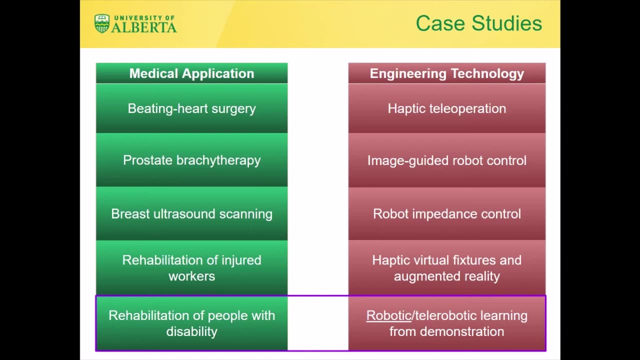 When a patient uses this system, quantitative assessments can be performed so that the therapist can best guide the patient through the next stages of rehabilitation. Yet another way to bring semi-autonomy into medical robotic systems is through machine learning, such that the robot can learn what it needs to do. 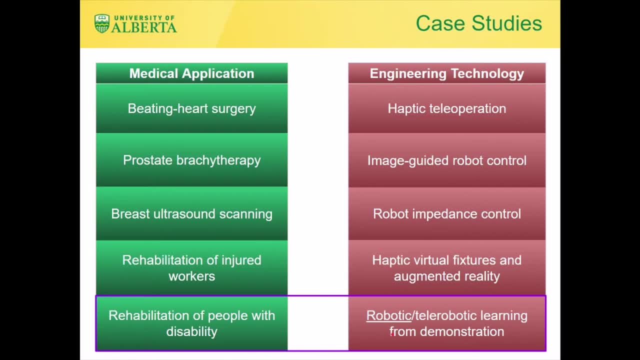 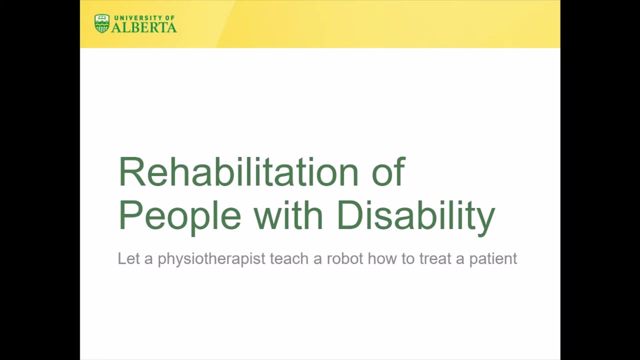 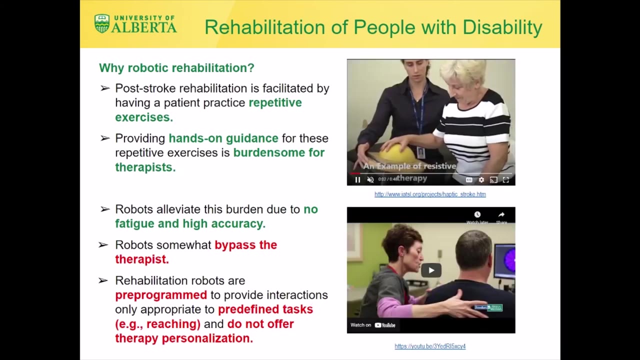 through hands-on kinesthetic teaching provided by a clinician For rehabilitation of people with disability. we can use machine learning in order to let a physiotherapist teach a robot how to treat a patient. Post-stroke rehabilitation is facilitated by having a patient practice repetitive exercises. 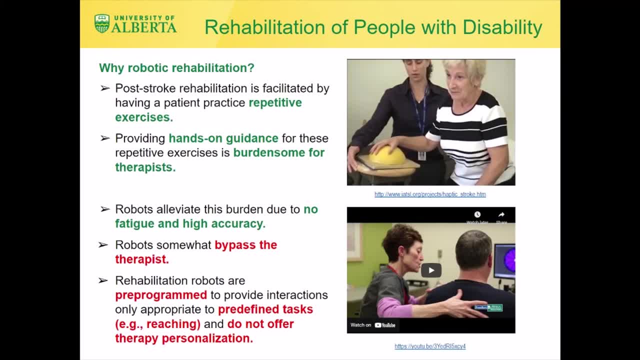 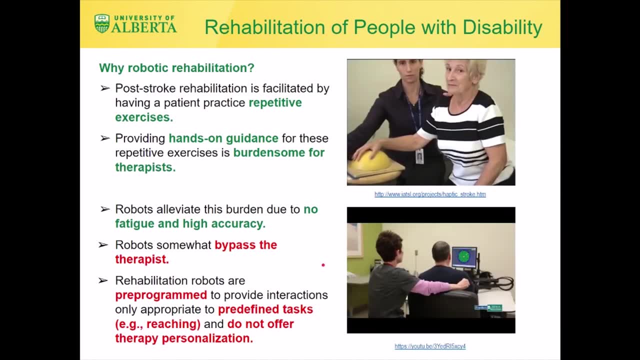 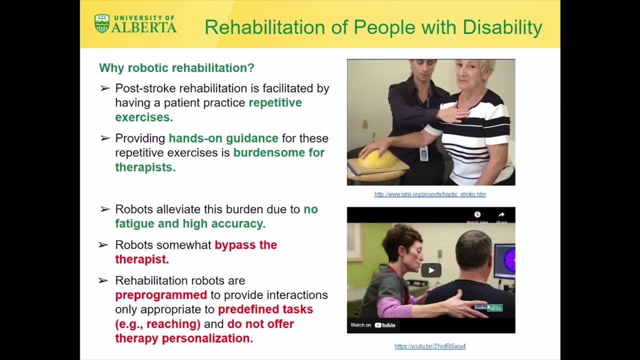 Providing hands-on guidance for these repetitive exercises is burdensome for therapists. Robots alleviate this burden, but then they may bypass the therapies and generally are pre-programmed to provide interactions only appropriate to predefined tasks. Incorporation of activities of daily living or ADLs. 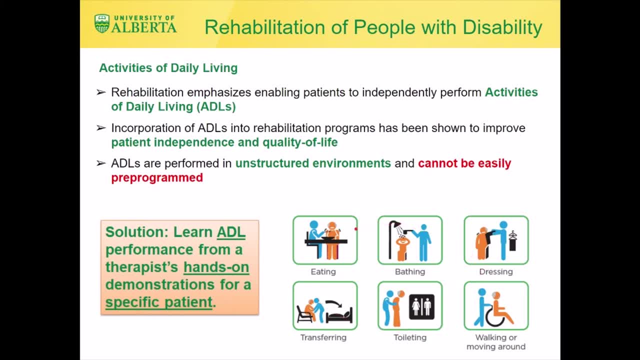 into rehabilitation programs has been shown to improve patient independence and quality of life. However, the issue is that ADLs are performed in unstructured environments and cannot be easily pre-programmed into robots. However, machine learning and semi-autonomy can offer a solution. 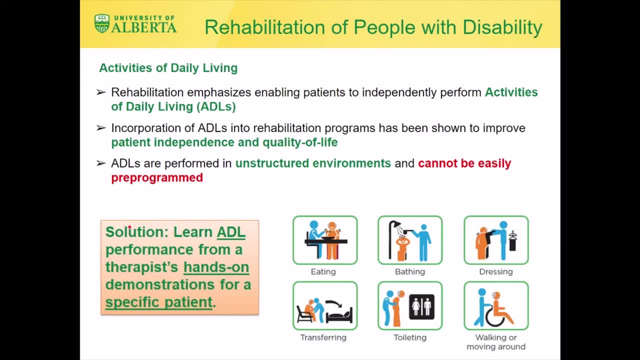 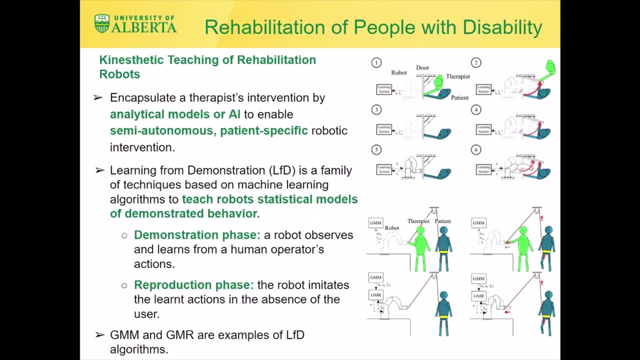 Learn an ADL performance from a therapist's hands-on demonstrations and reproduce the same later in the absence of the therapist. This makes it possible to encapsulate a therapist's intervention by analytical models or AI to enable semi-autonomous, patient-specific robotic intervention In the demonstration phase. 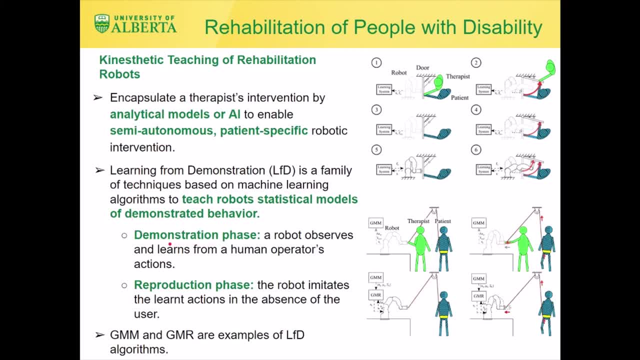 a robot observes and learns from a therapist's actions what it is supposed to do for a given patient. Later, and in the reproduction phase, the robot imitates the learned actions in the absence of the therapist so that the patient can continue with the task. 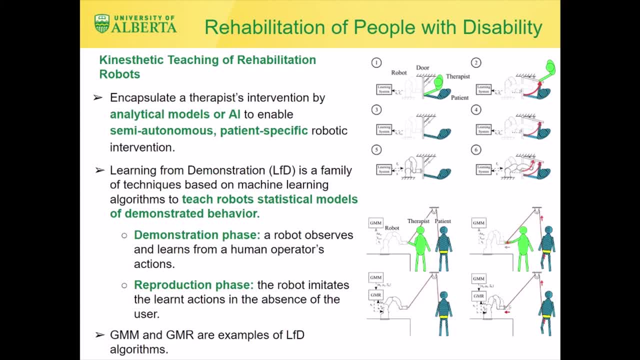 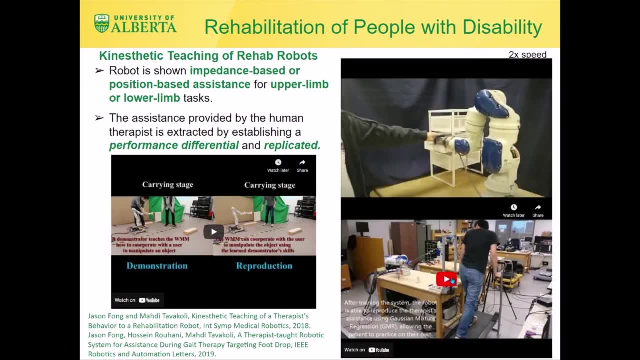 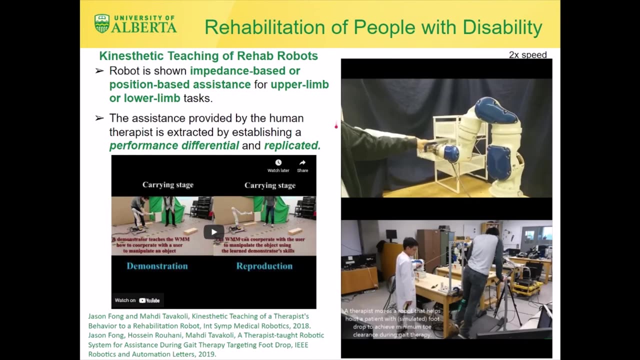 and therefore receive a higher dose of rehabilitation exercises than normally possible. Here the temporal separation of autonomy between a clinician and a robot is shown for several tasks. First, a robot is shown an impedance-based or position-based assistance by the therapist for upper limb or lower limb tasks. 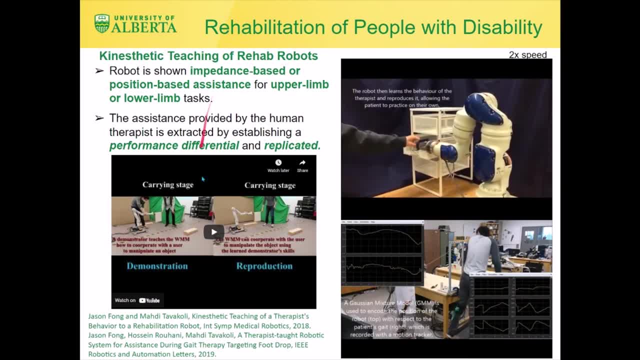 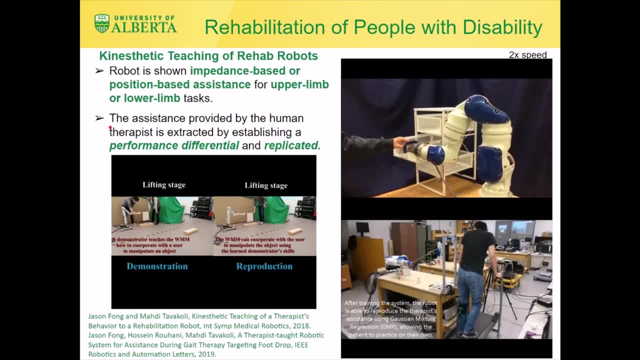 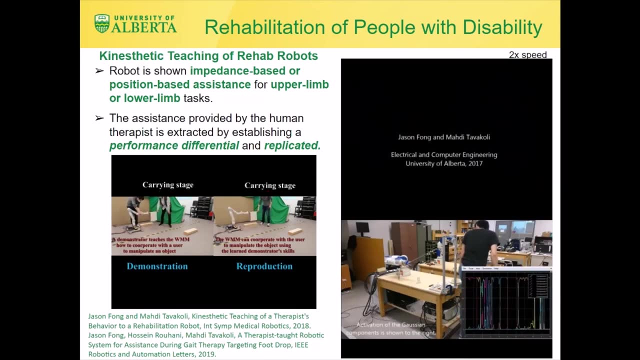 Then the assistance that was provided by the therapist is extracted using machine learning and replicated robotically so that the patient can continue to receive the same assistance in the absence of the therapist. The left-hand side video shows the same: for a cooperative objective, think task. 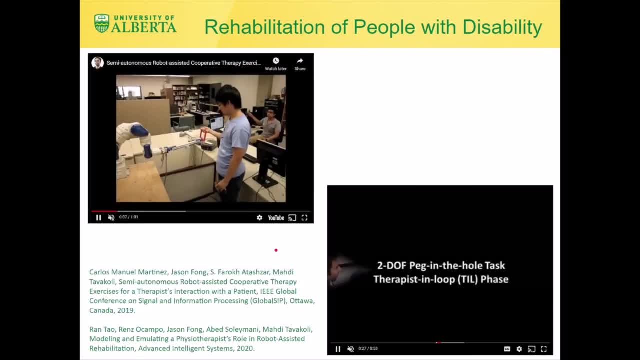 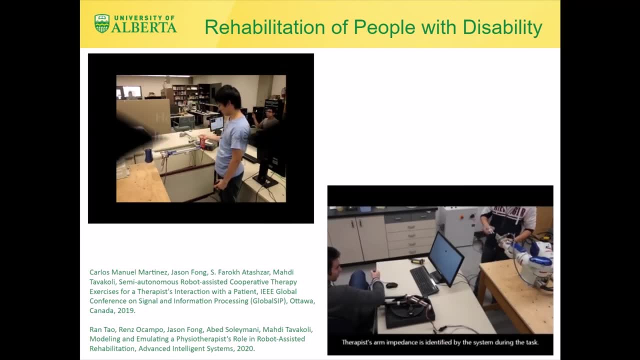 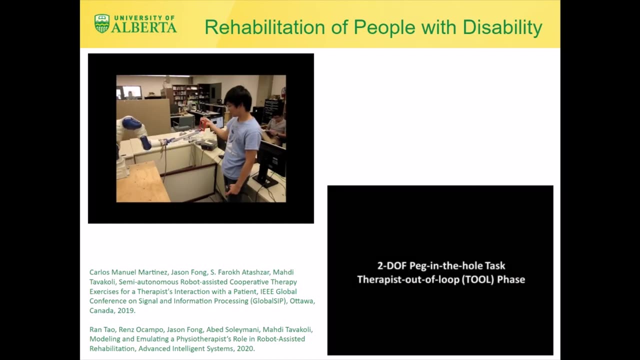 The idea of sharing control on a temporal basis using robot learning and intelligence can be implemented also over a long distance to enable tele-assessment and tele-rehabilitation. For a short time period, a physiotherapist intervenes kinesthetically to assist the user in the performance of a two-user task. 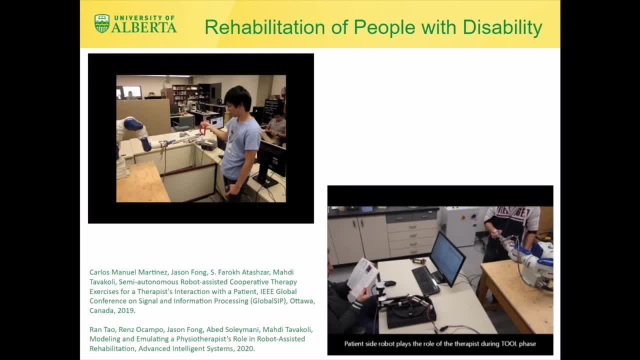 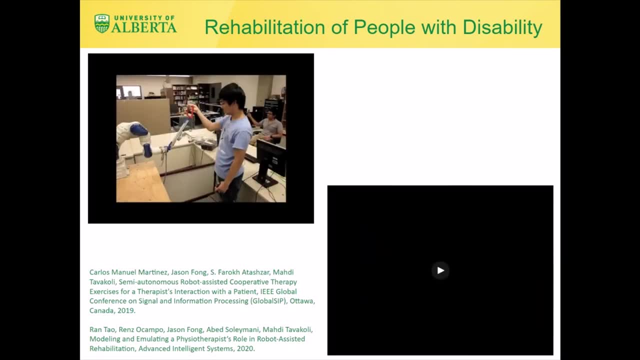 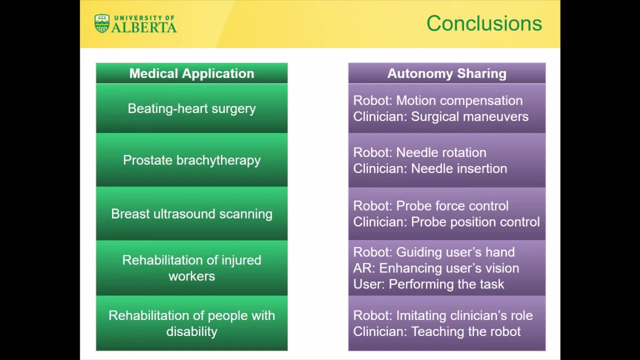 The behavior demonstrated by the therapist is captured by AI and reproduced robotically so that the user has more opportunities to do the same exercises in the absence of the therapist. These are several ways to use intelligent control and AI to share autonomy between a clinician and a robot. 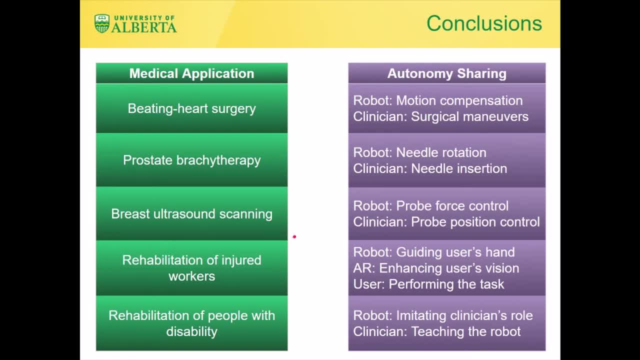 for reduced workload for the clinicians and improved outcomes for the patients. Depending on the application, the robot can take care of tasks beyond the sensory motor capabilities of the clinician, Tasks that require image processing, measurement and computation Tasks that cause fatigue for the clinician. 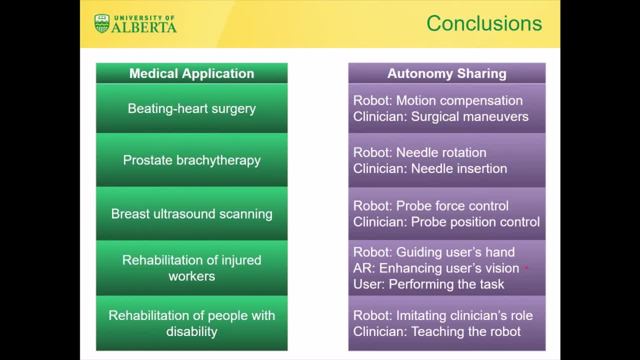 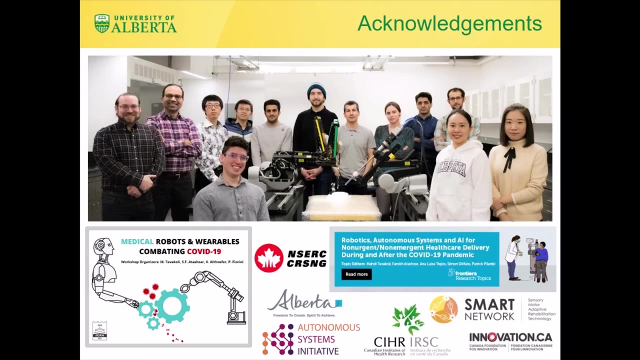 or have low repeatability, Tasks where the user can benefit from haptic guidance or augmented vision, And tasks that can be learned based on a clinician's hands-on demonstration and reproduced later, such that the patient can have increased access to healthcare. Thank you all very much for your time.